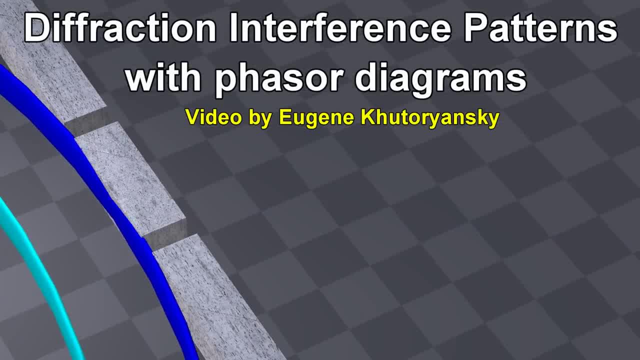 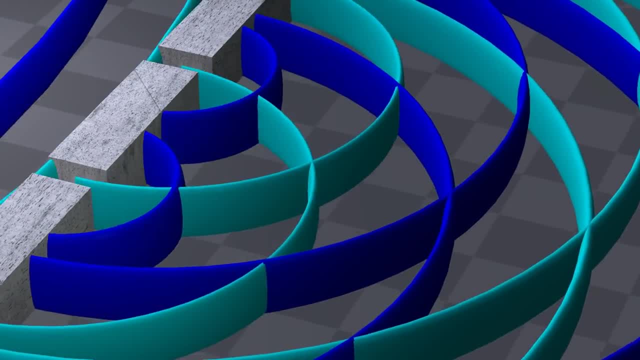 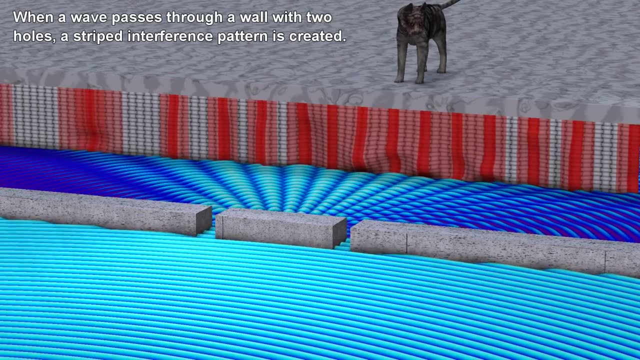 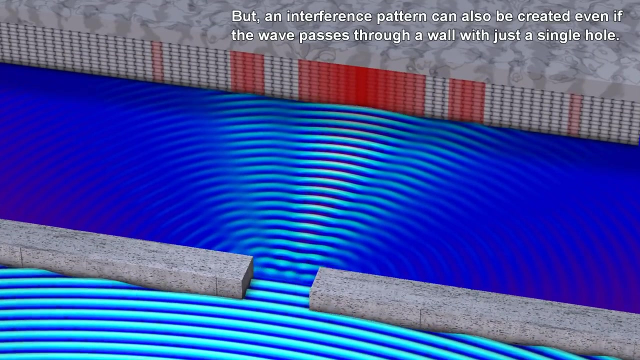 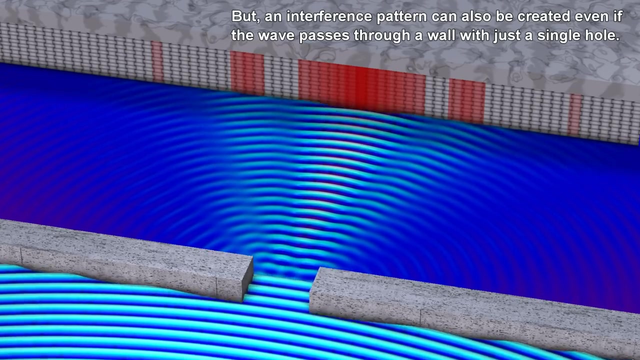 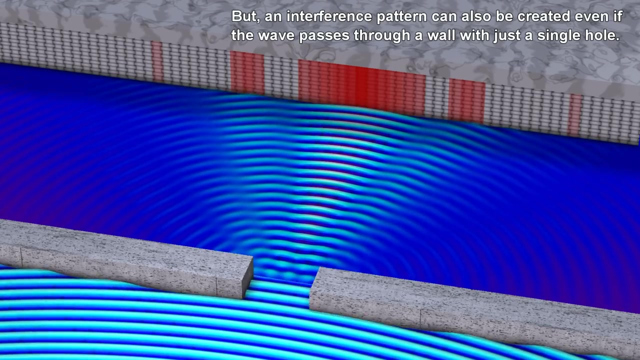 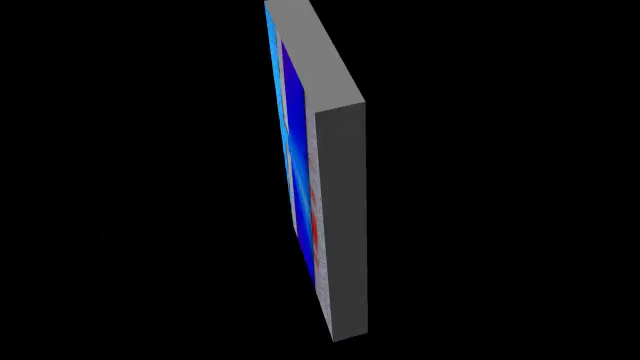 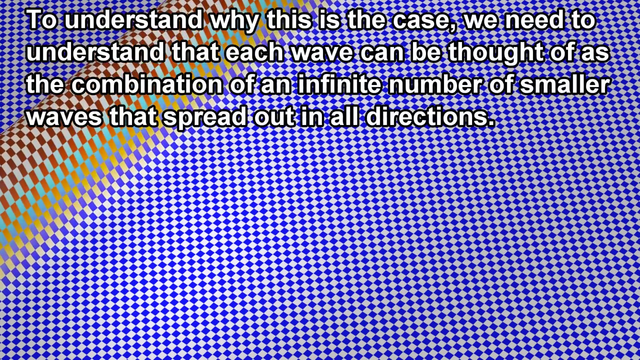 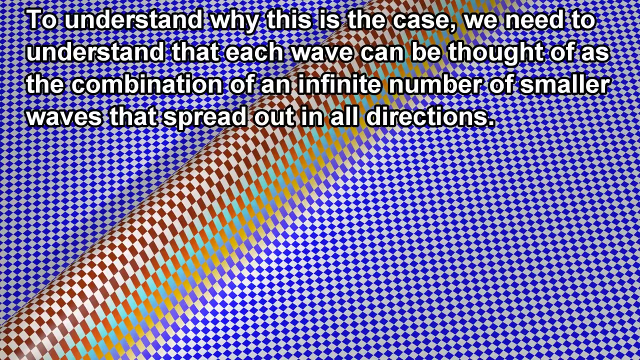 When a wave passes through a wall with two holes, a striped interference pattern is created, But an interference pattern can also be created even if the wave passes through a wall with just a single hole. To understand why this is the case, we need to understand that each wave can be thought of as the combination of an infinite number of smaller waves that spread out in all directions. 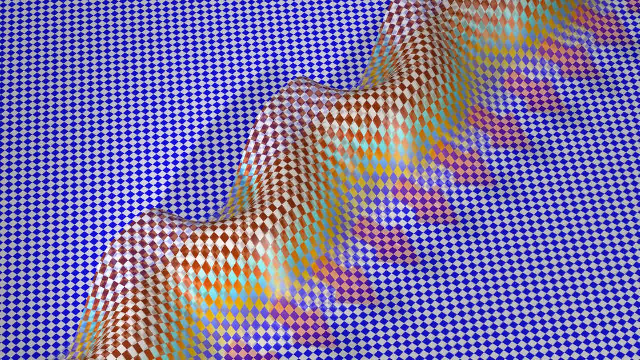 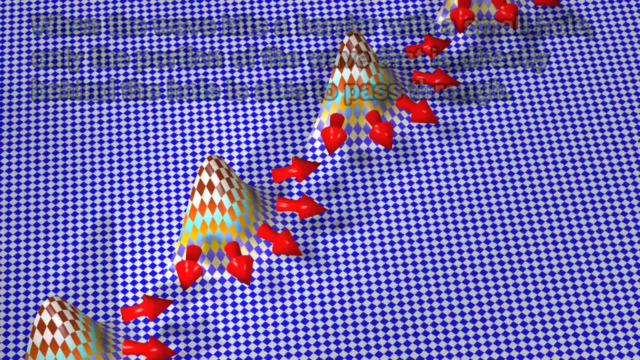 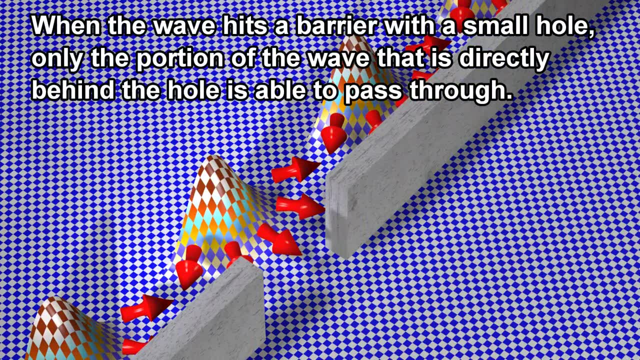 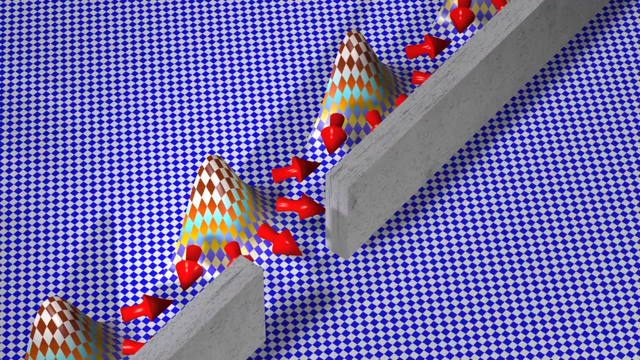 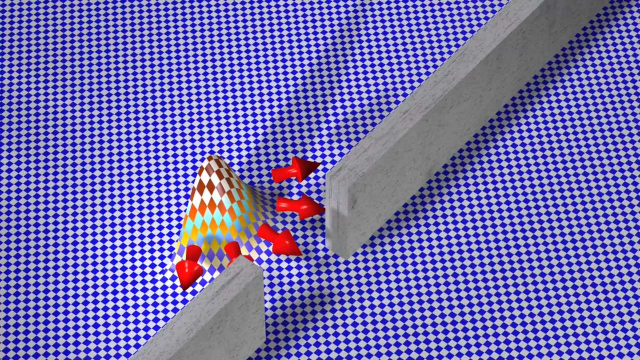 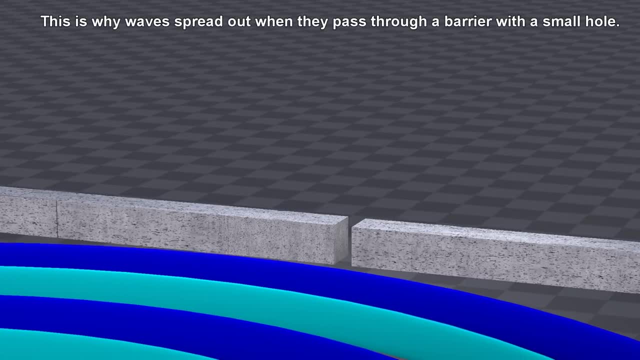 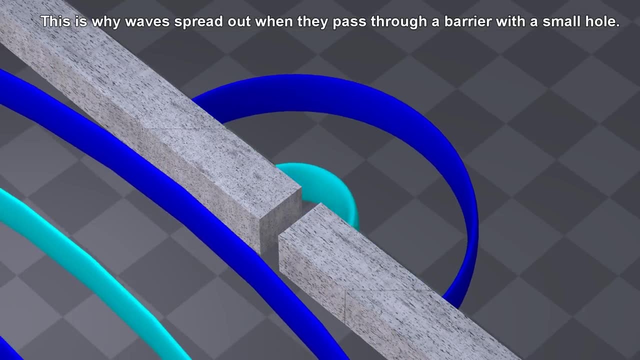 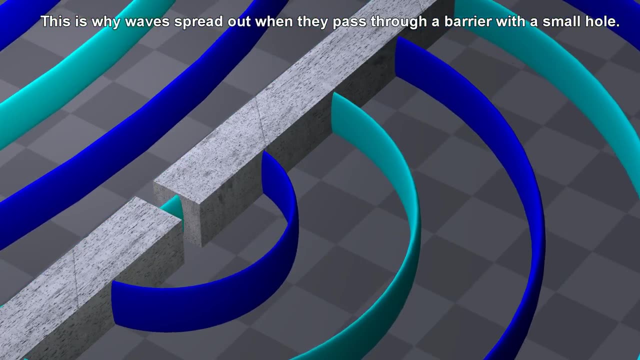 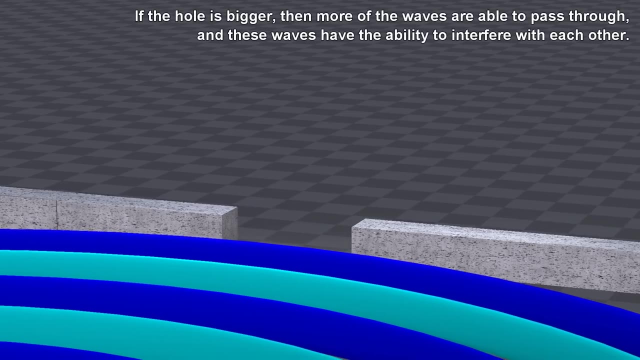 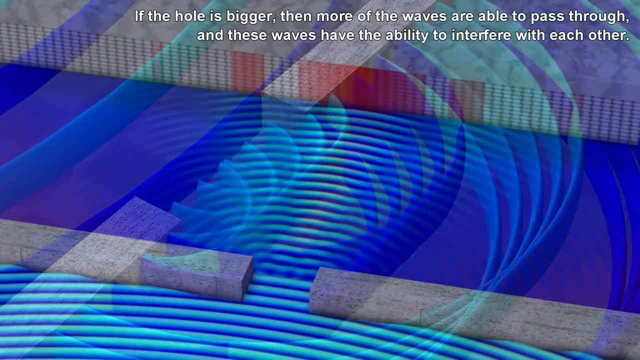 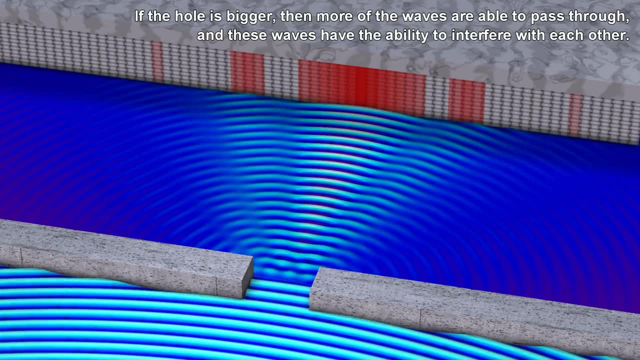 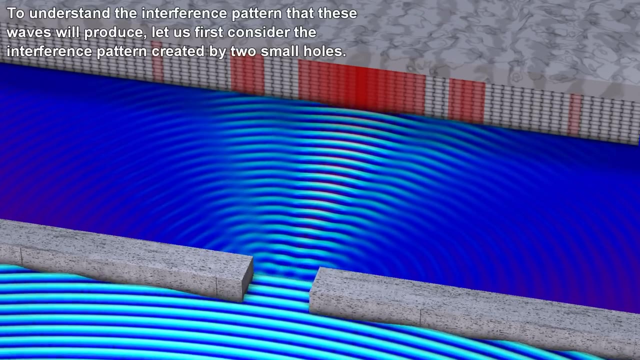 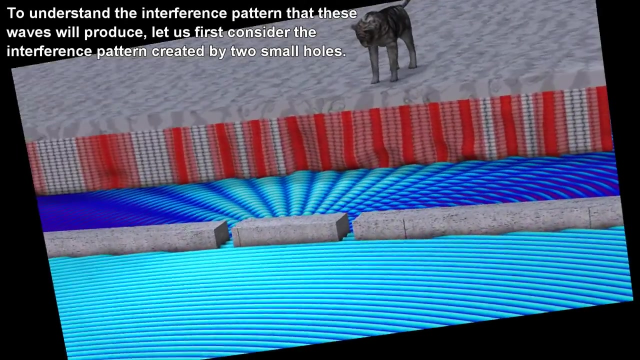 If the whole of the wave is a barrier, only the portion of the wave that is directly behind the hole is able to pass through. To understand the interference pattern that these waves will produce, let us first consider the interference pattern created by two small holes. 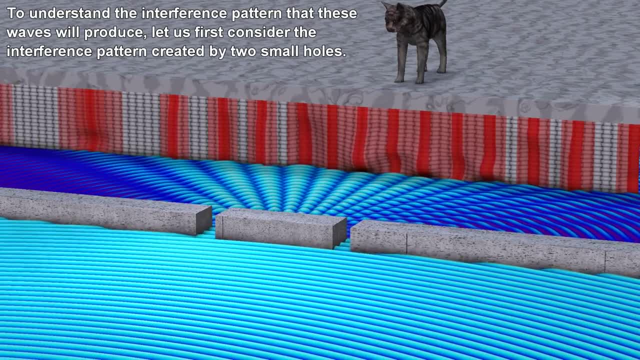 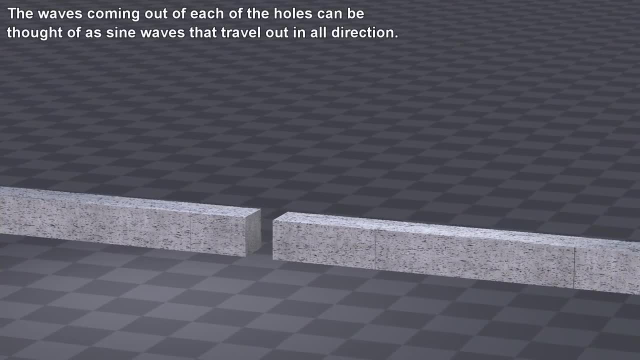 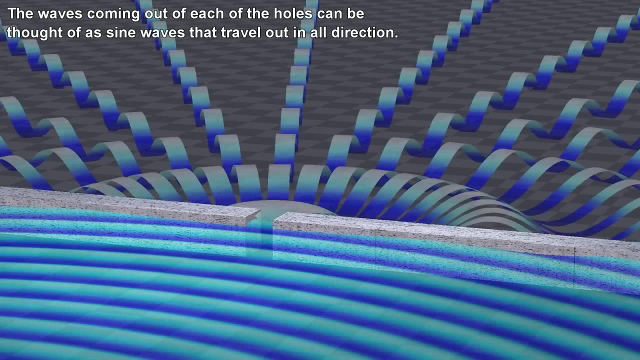 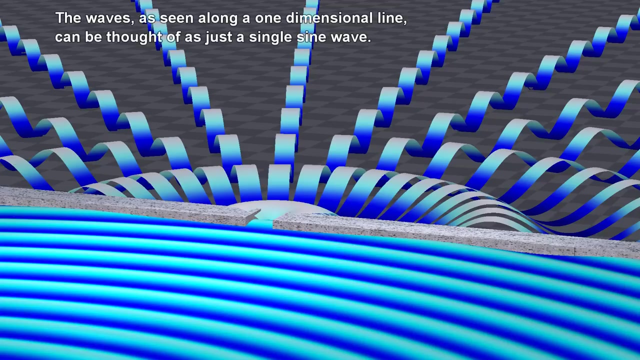 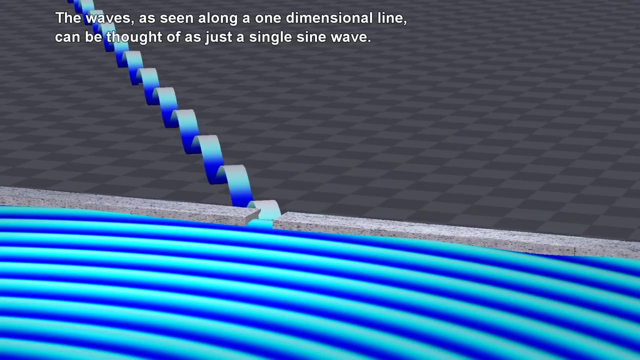 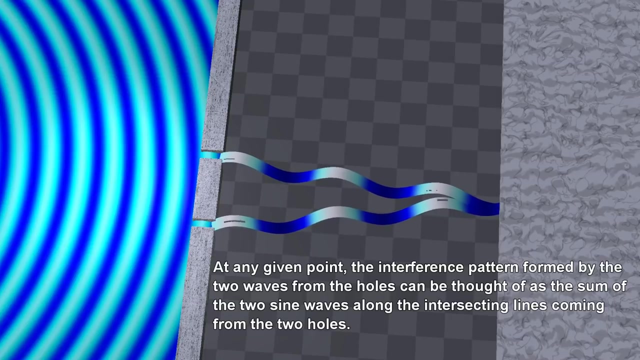 The waves coming out of each of the holes can be thought of as sine waves that travel out in all directions. The waves as seen along a one-dimensional line can be thought of as just a single sine wave At any given point. the interference pattern formed by the two waves from the 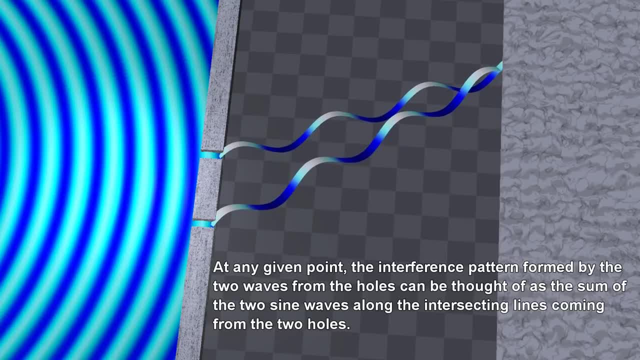 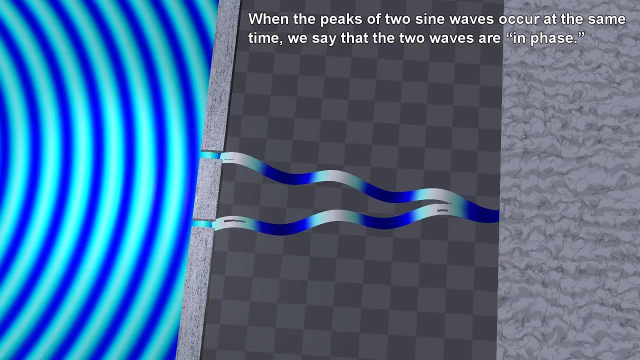 two holes can be thought of as the sum of the two sine waves along the intersecting lines coming from the two holes. When the peaks of two sine waves occur at the same time, we say that the two waves are in phase, Since both sine waves are created by the same original wave which passes through both holes. 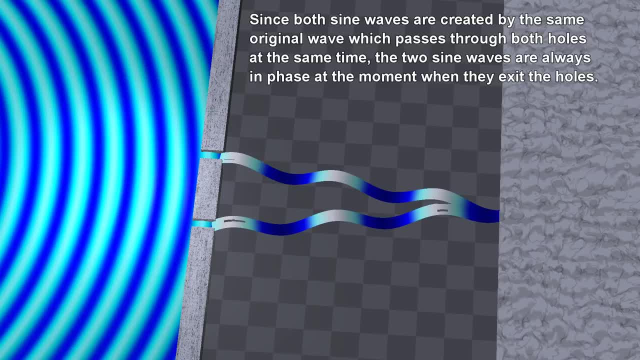 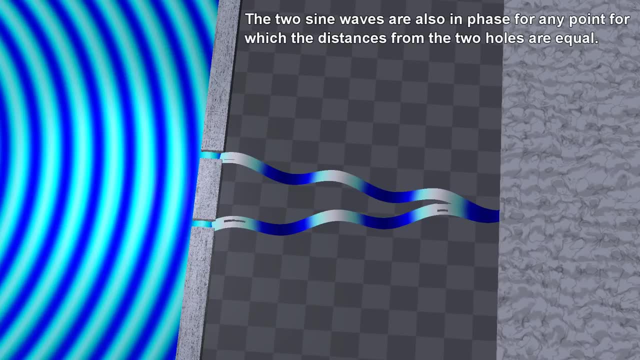 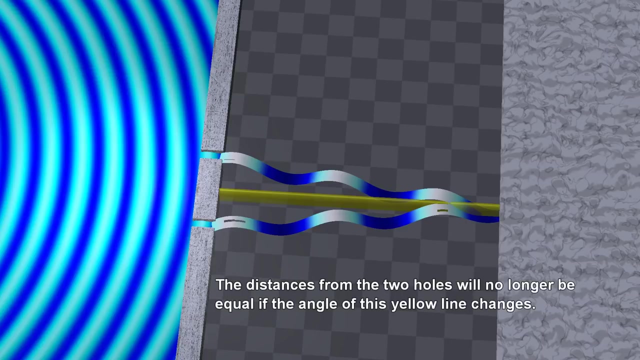 at the same time. the two sine waves are always in phase at the moment when they exit the holes. The two sine waves are also in phase for any point for which the distances from the two holes are equal. The distances from the two holes will no longer be equal if the angle of this yellow line 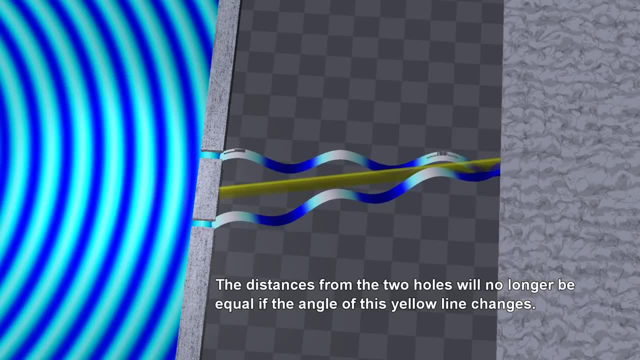 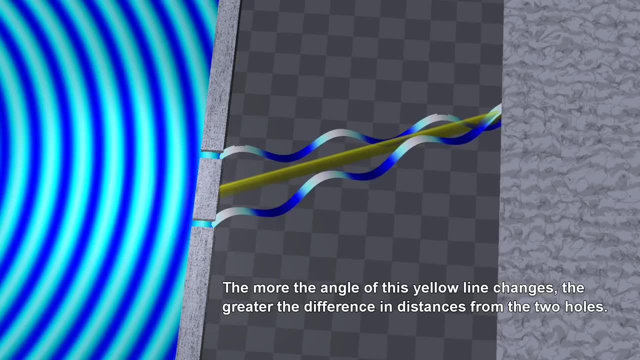 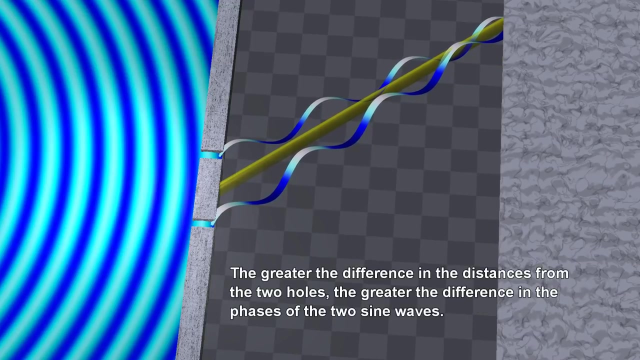 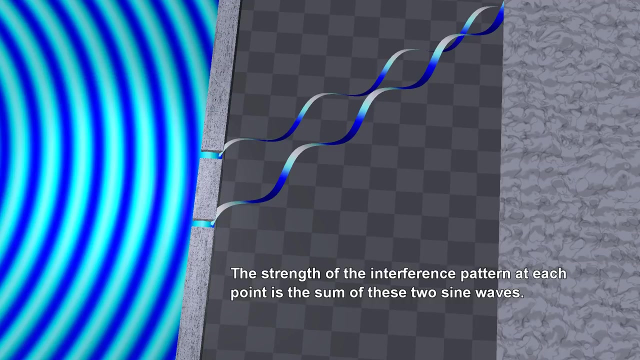 changes. The more the angle of this yellow line changes, the greater the difference in distances from the two holes. The greater the difference in the distances from the two holes, the greater the difference in the phases of the two sine waves. The strength of the interference pattern at each point is the sum of these two sine waves. 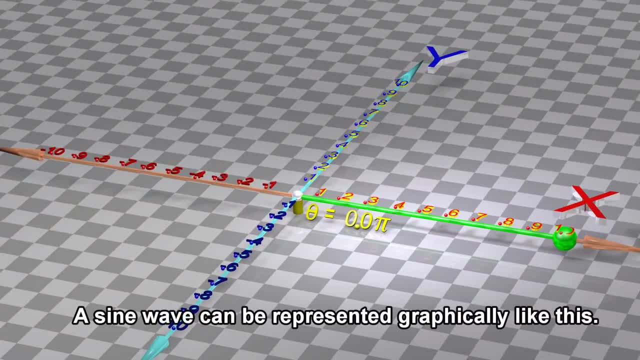 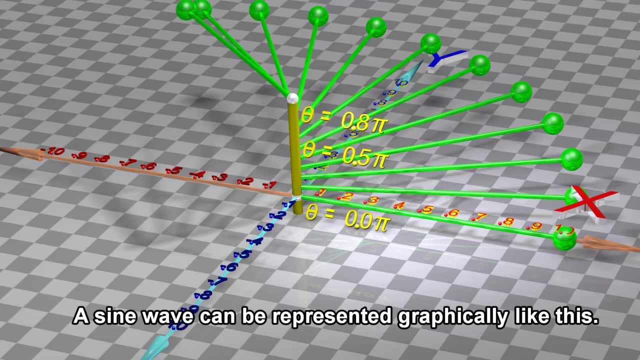 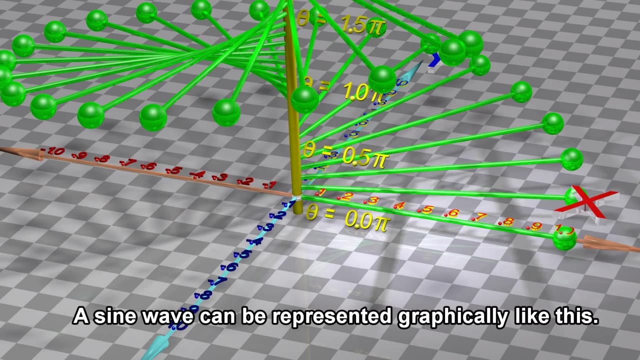 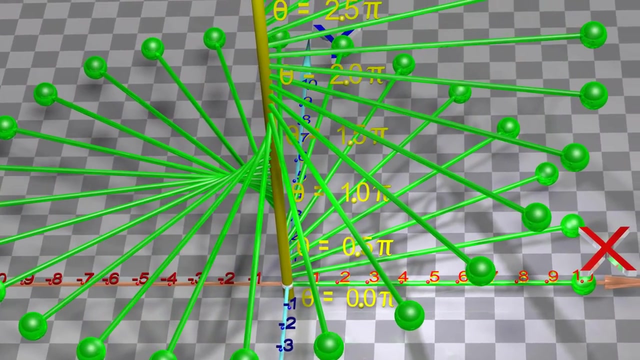 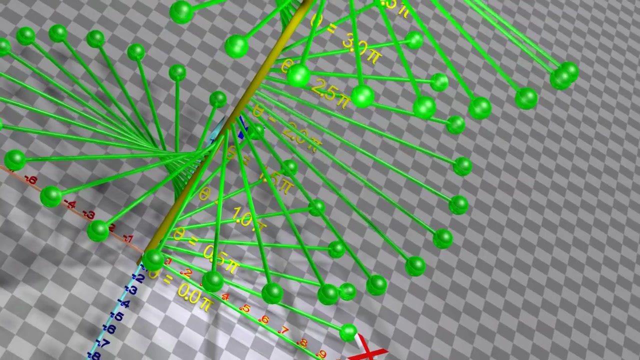 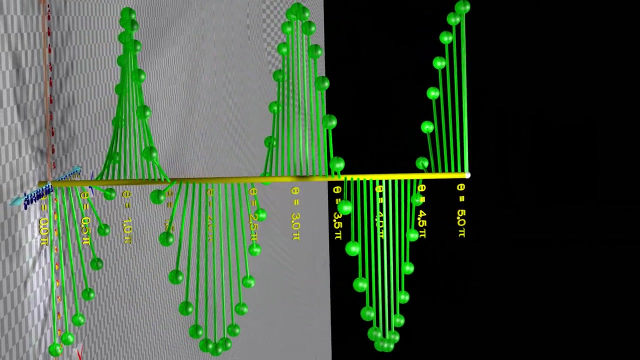 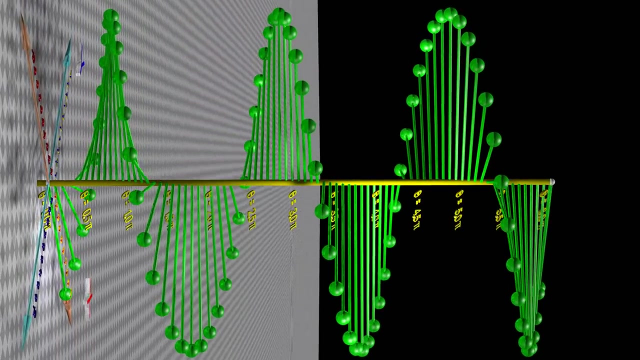 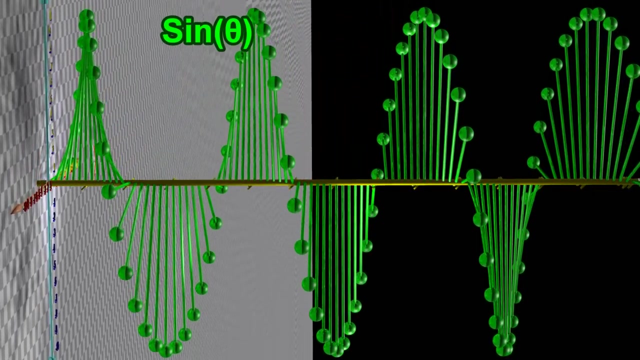 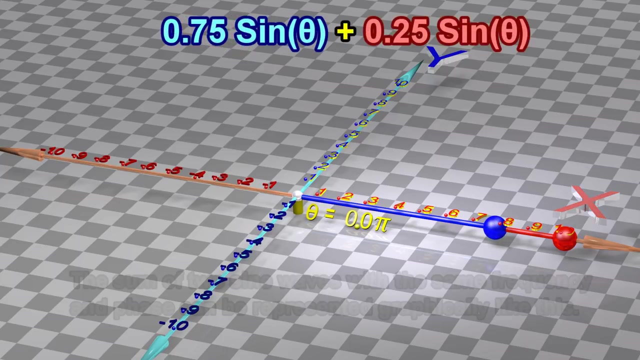 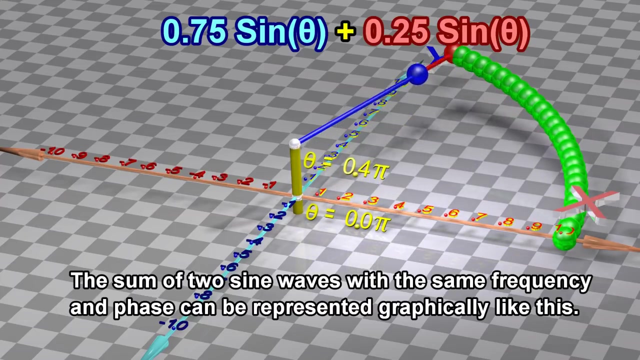 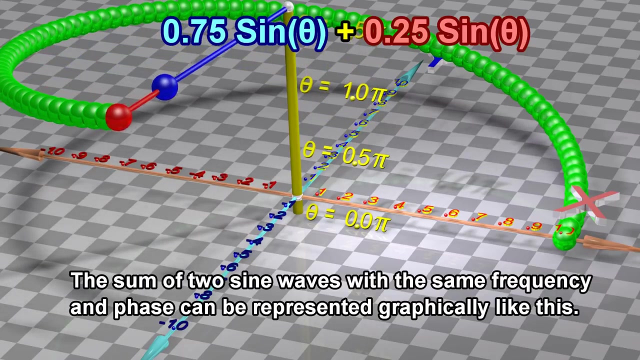 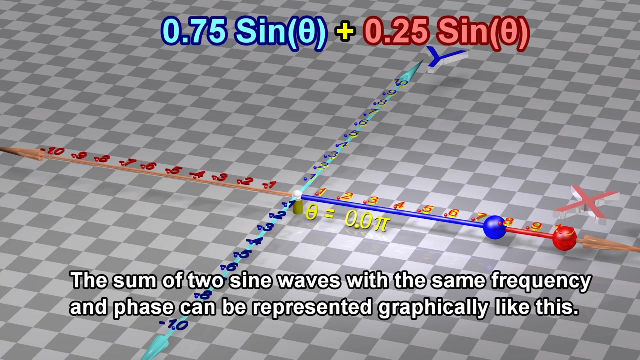 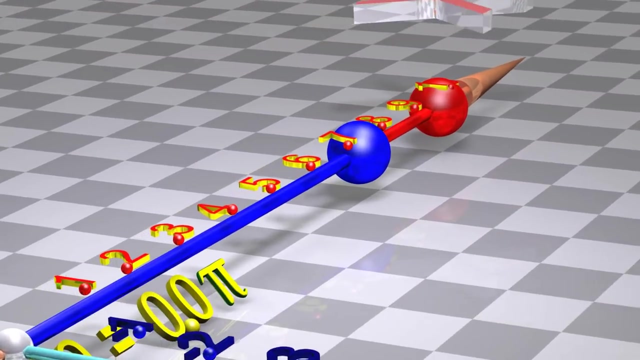 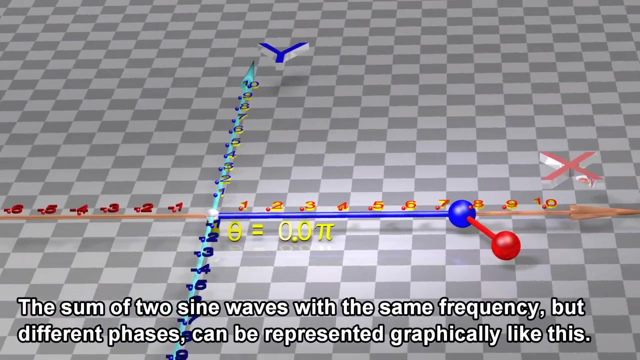 A sine wave can be represented graphically like this: The sine wave can be represented graphically like this: The sum of two sine waves with the same frequency and phase can be represented graphically like this: The sum of two sine waves with the same frequency but different phases can be represented graphically like this: 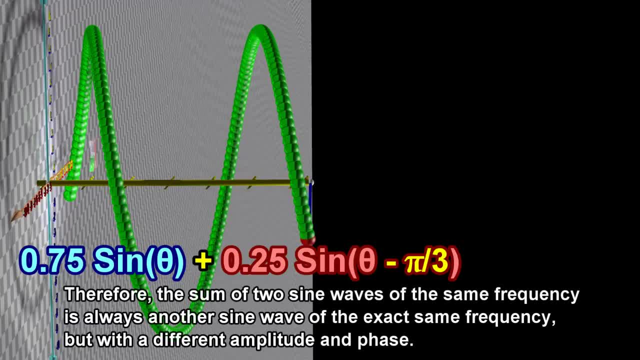 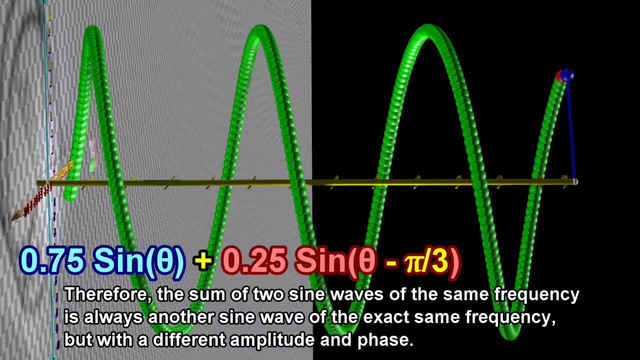 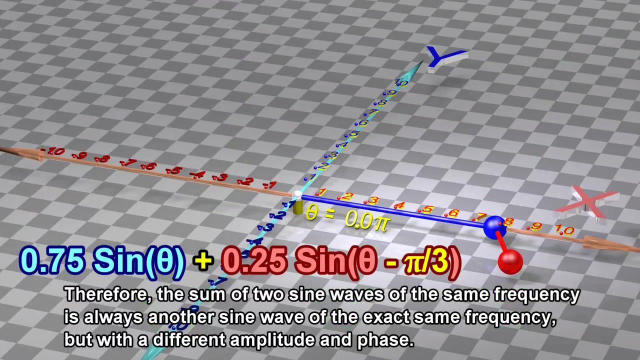 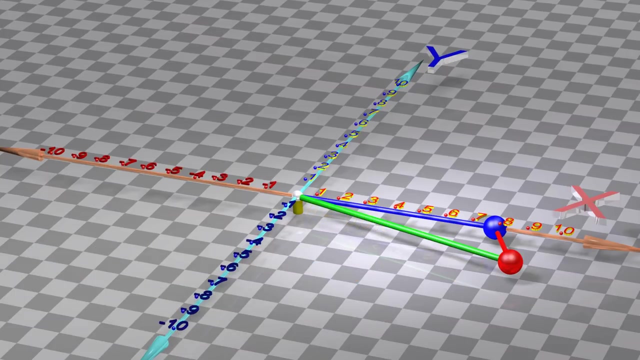 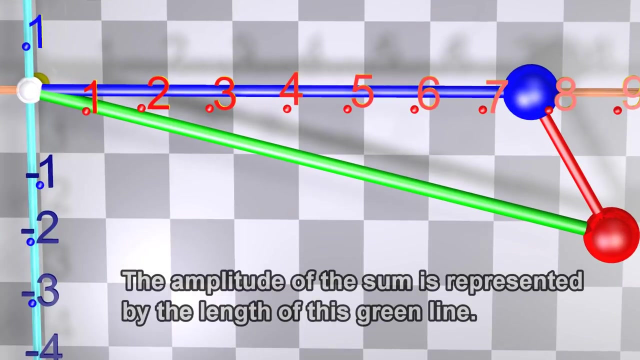 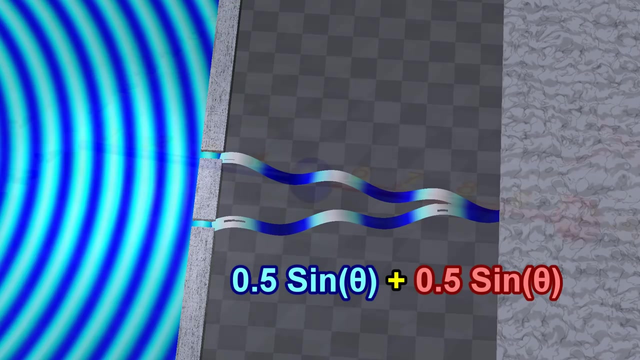 Therefore, the sum of two sine waves of the same frequency is always another sine wave of the exact same frequency, but with a different amplitude and phase. The amplitude of the sum is represented by the length of this green line In the case of the sine waves coming from our two small holes. 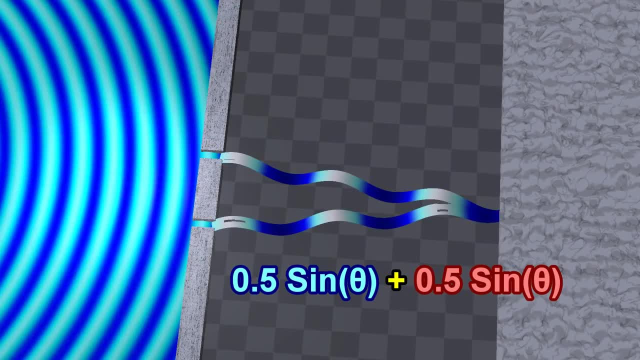 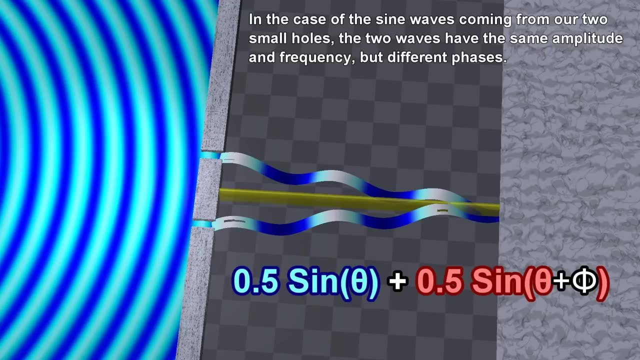 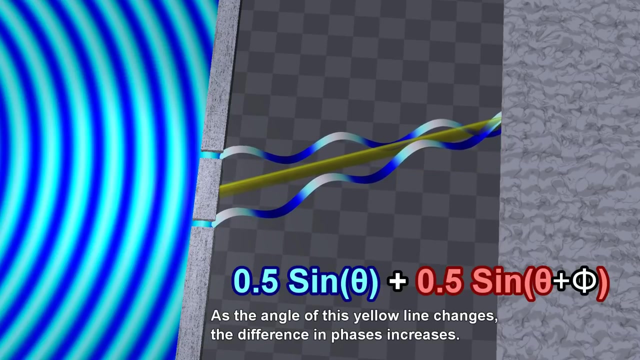 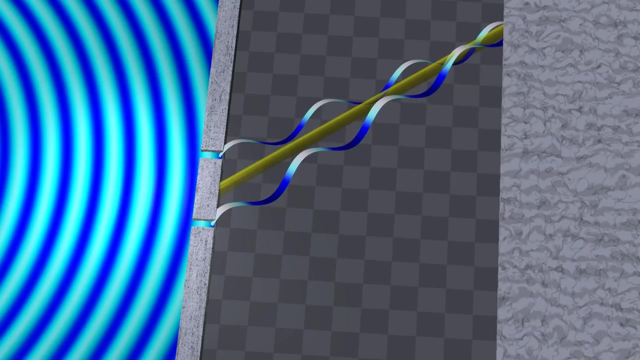 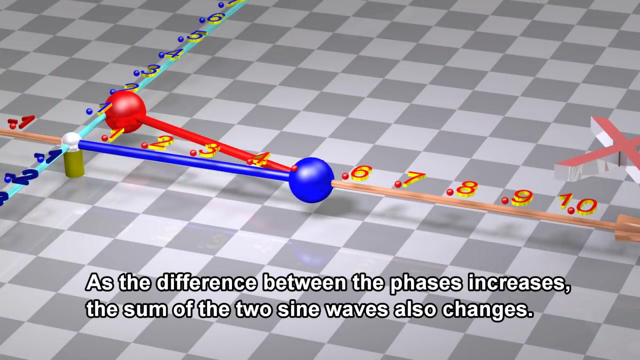 the two waves have the same amplitude and frequency, but different phases, As the angle of this yellow line is represented by the length of this green line. as the angle of this green line changes, the difference in phases increases. As the difference between the phases increases, the sum of the two sine waves also changes. 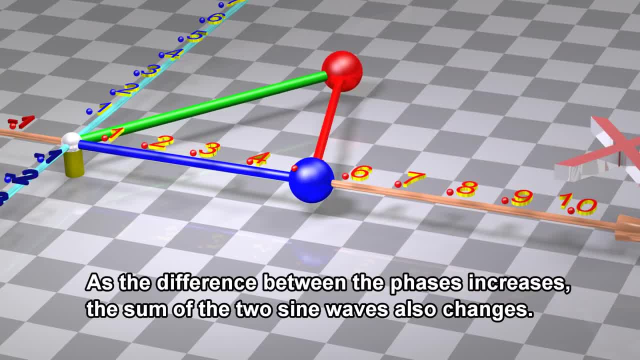 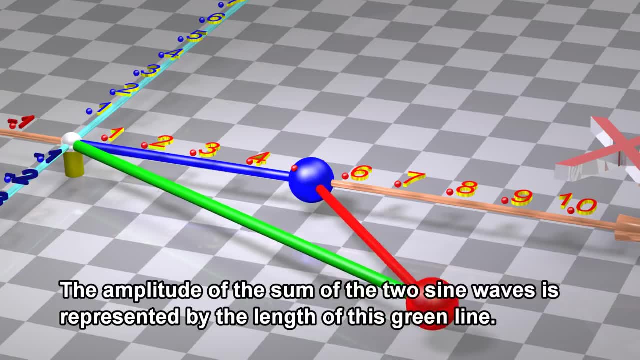 The amplitude of the sum of the two sine waves is represented by the length of this green line. The amplitude of the sum of the two sine waves is represented by the length of this green line. In some cases, their sum has a very large amplitude. 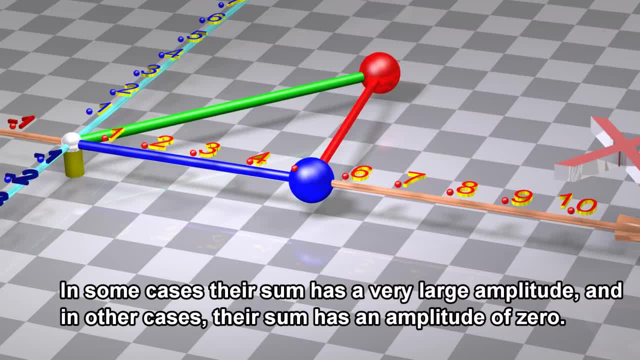 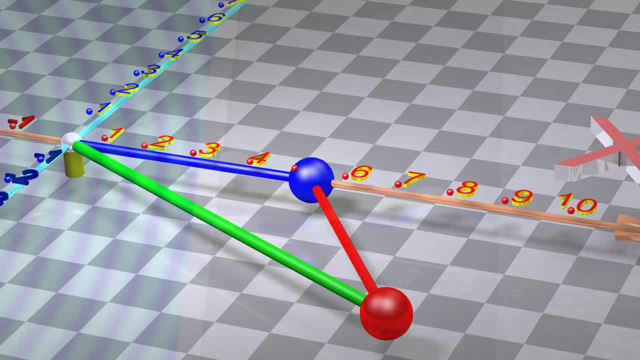 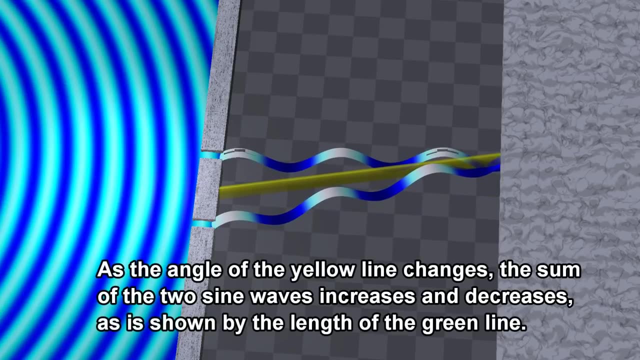 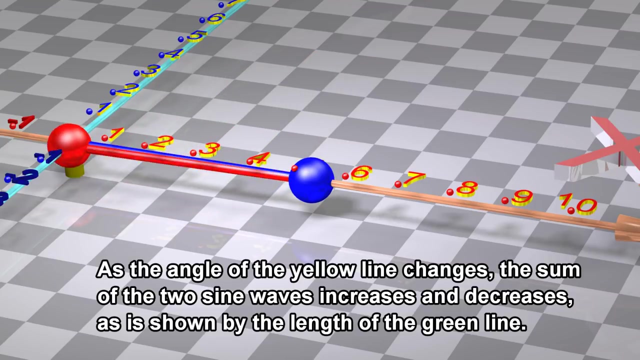 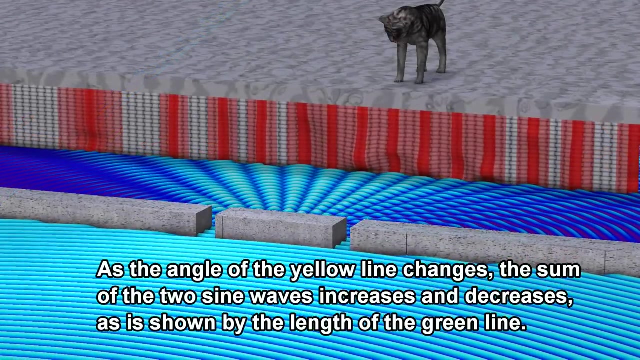 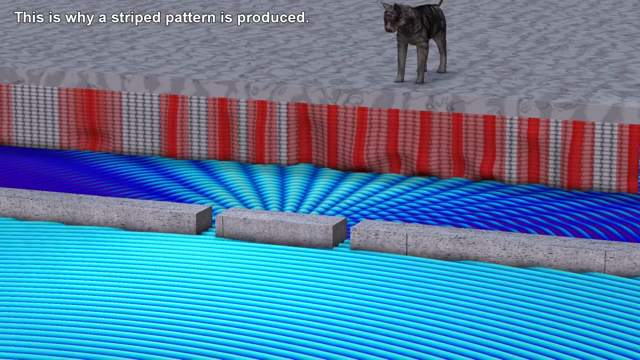 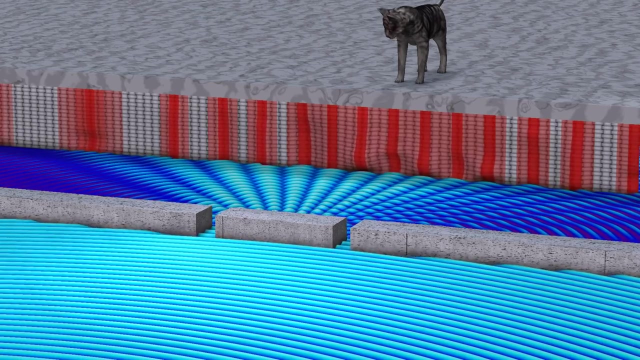 and in other cases their sum has an amplitude of zero. As the angle of the yellow line changes, the sum of the two sine waves increases and decreases, as is shown by the length of the green line. This is why a striped pattern is produced. 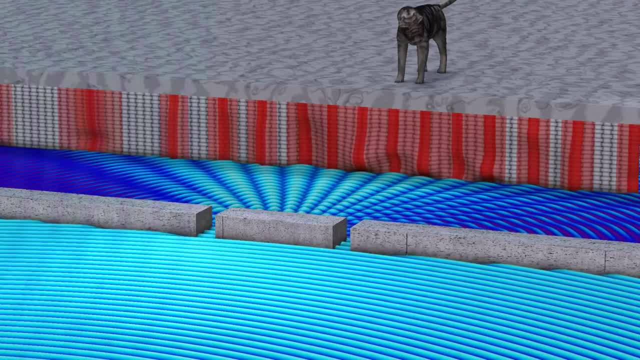 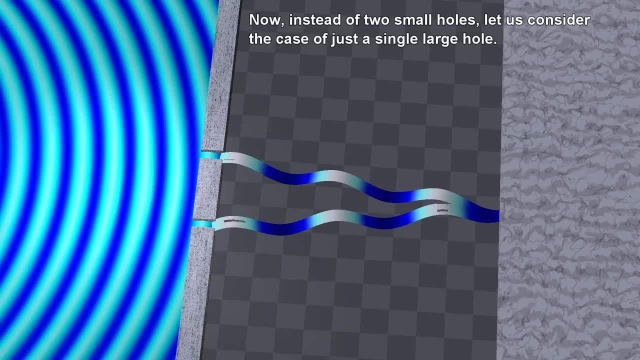 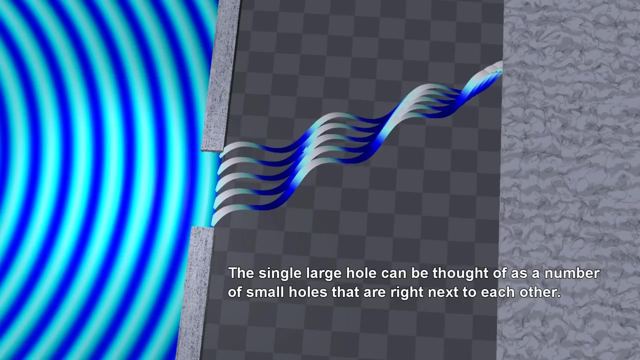 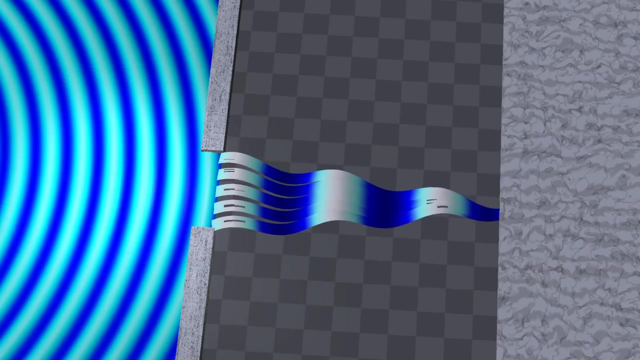 Now, instead of two small holes, let us consider the case of just a single large hole. The single large hole can be thought of as a number of small holes that are right next to each other. A sine wave comes out of each of these holes, and these sine waves add together. 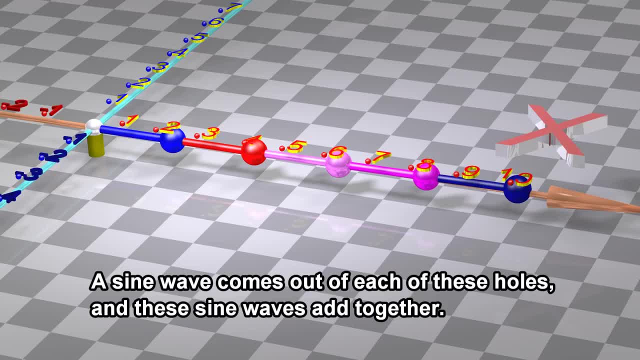 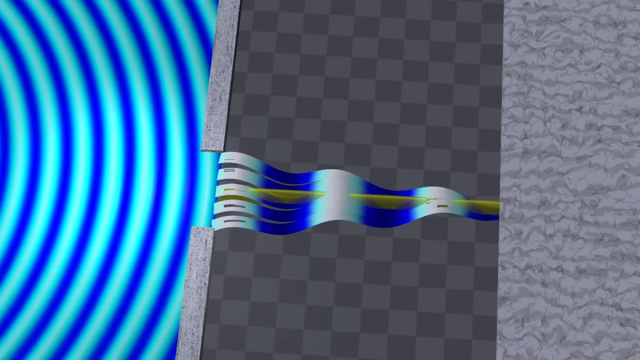 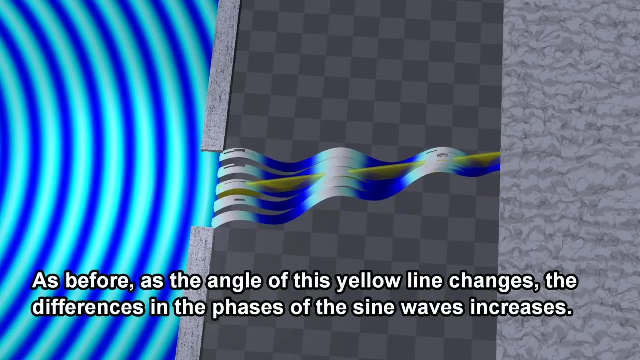 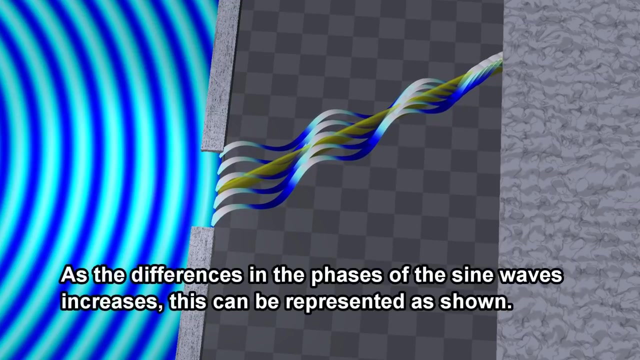 As before, as the angle of this yellow line changes, the differences in the phases of the sine waves increases. As before, as the angle of this yellow line changes, the differences in the phases of the sine waves increases. As before. as the angle of this yellow line changes, the differences in the phases of the sine waves increases. 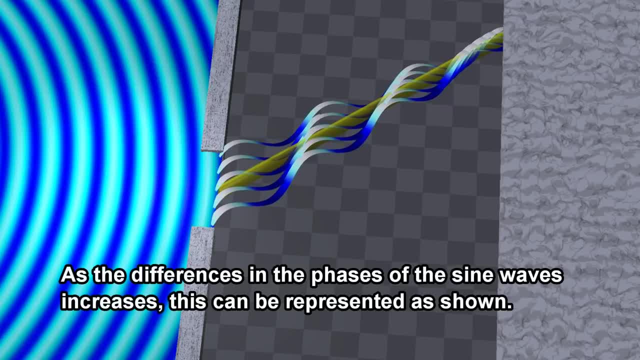 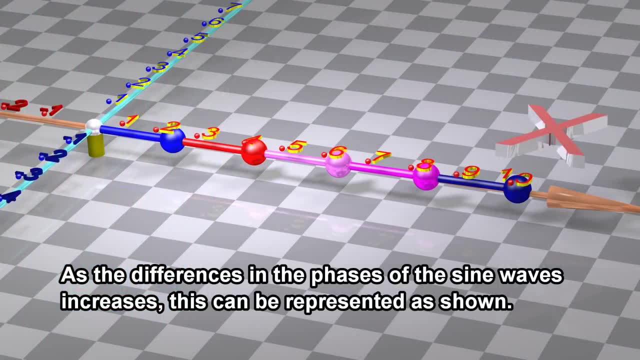 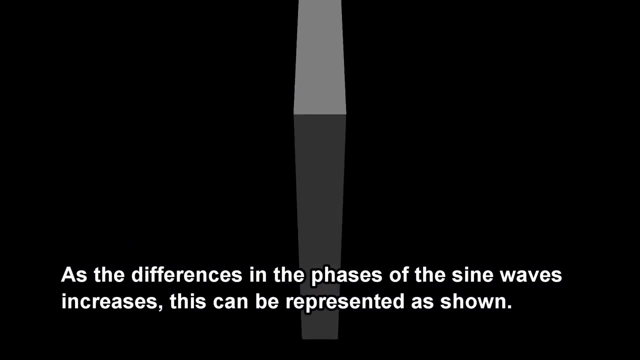 As the differences in the phases of the sine waves increases. this can be represented as shown: As before, as the angle of this yellow line changes, the differences in the phases of the sine waves increases. As before, as the angle of this yellow line changes, the differences in the phases of the sine waves increases. 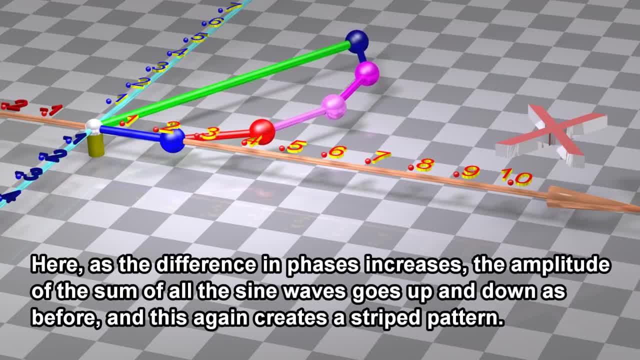 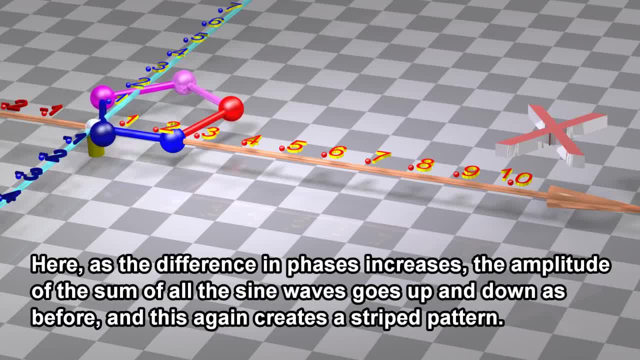 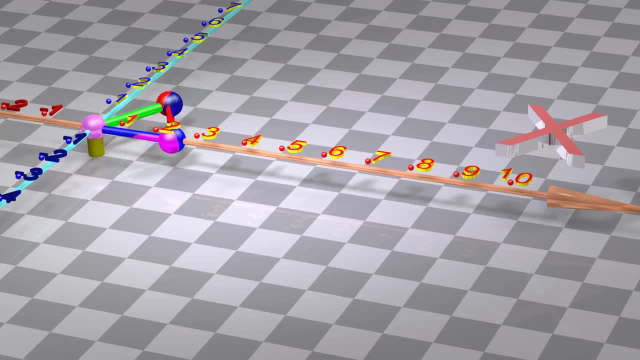 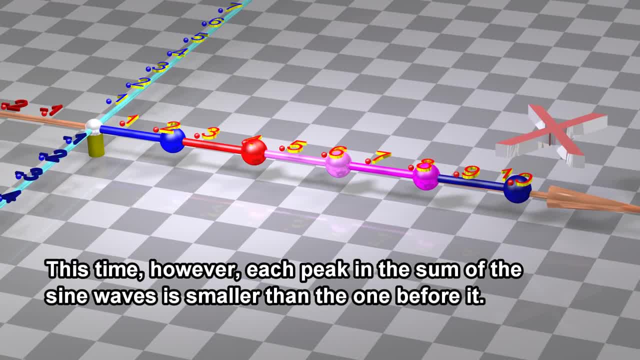 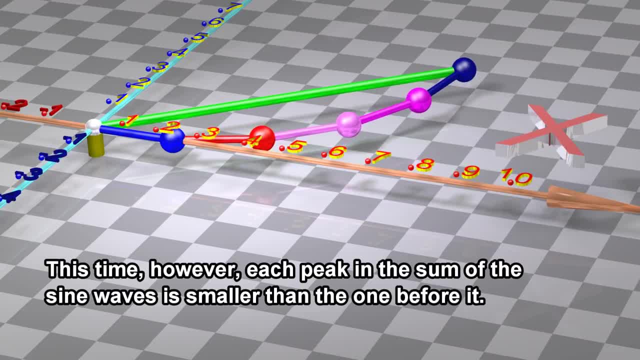 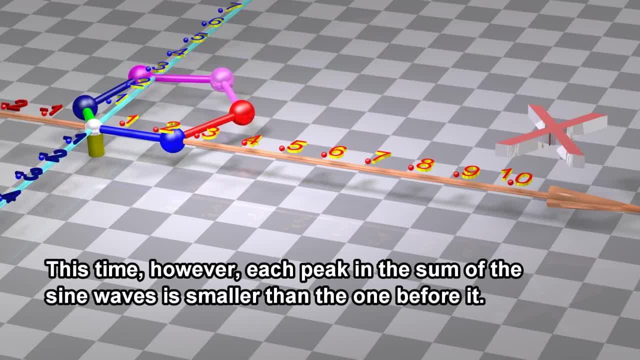 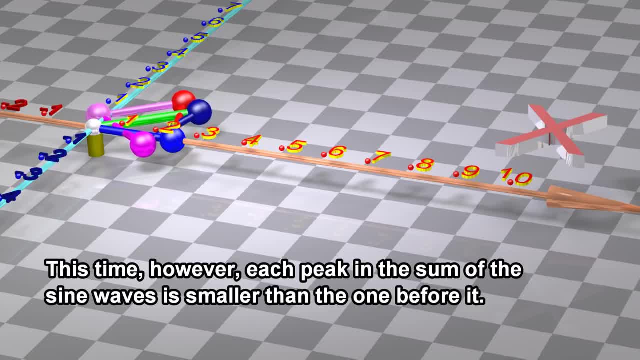 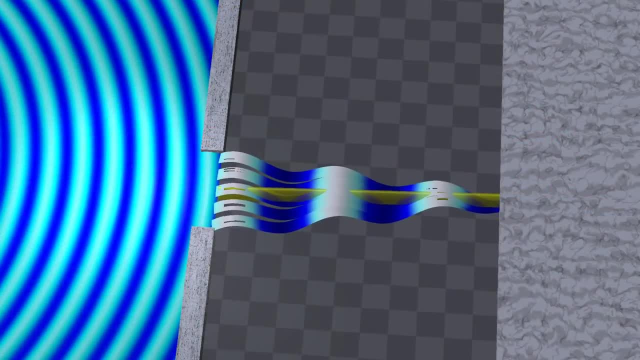 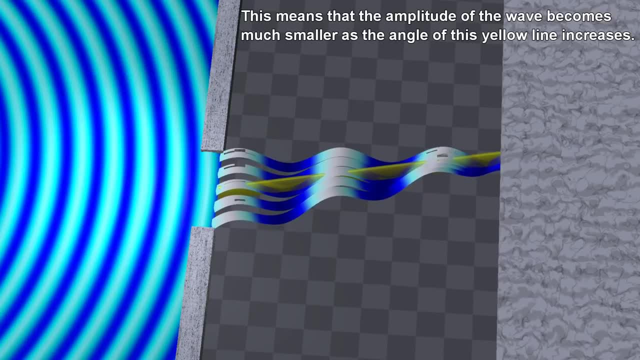 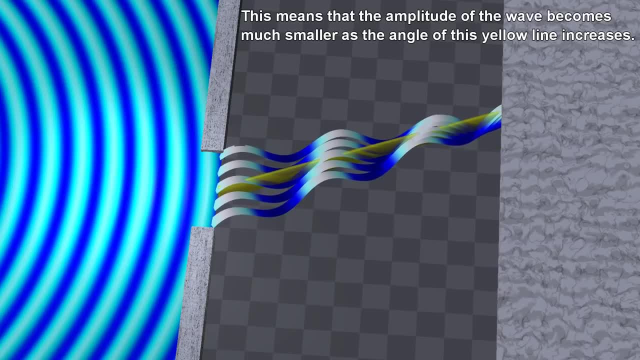 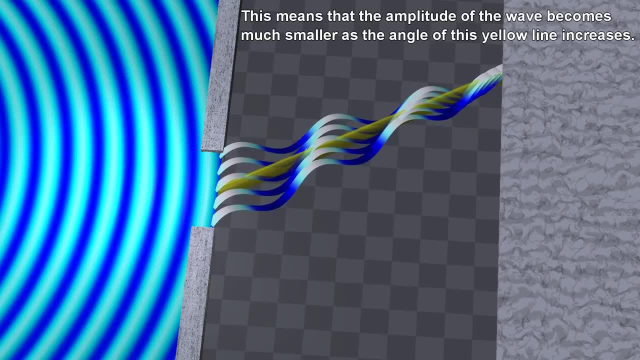 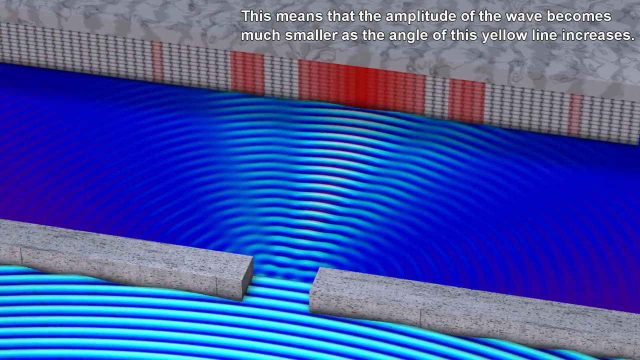 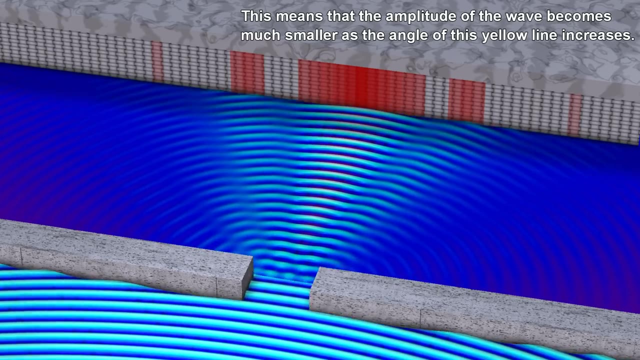 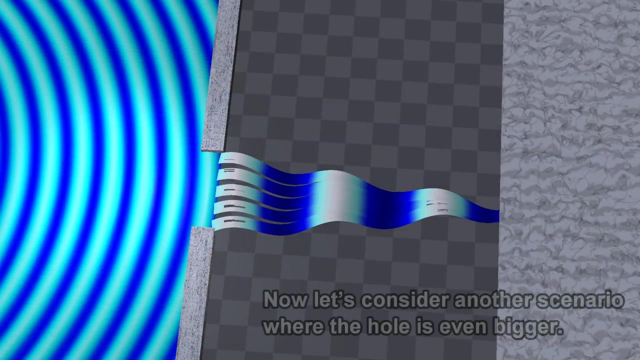 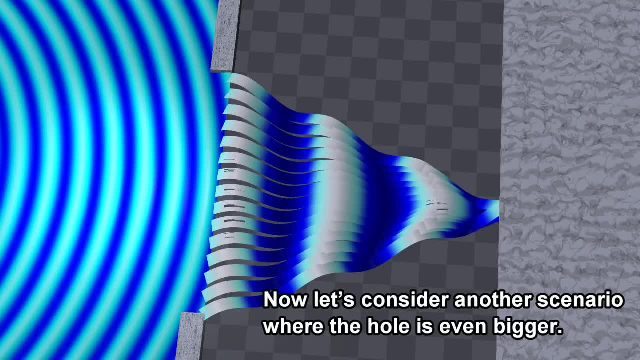 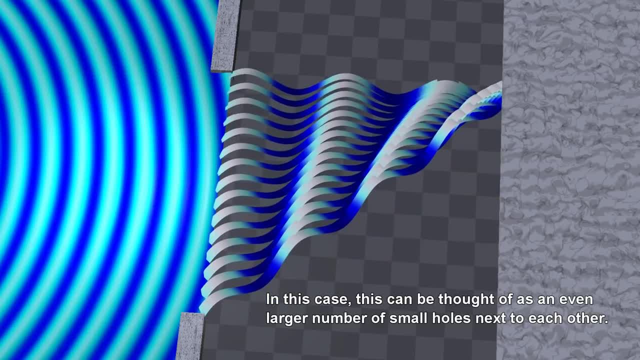 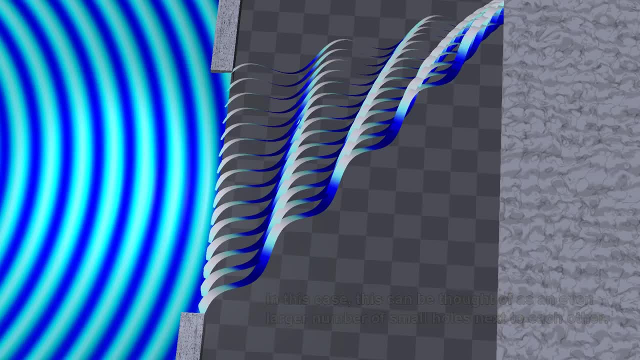 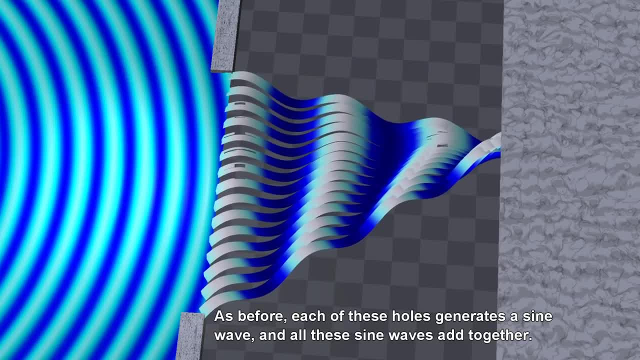 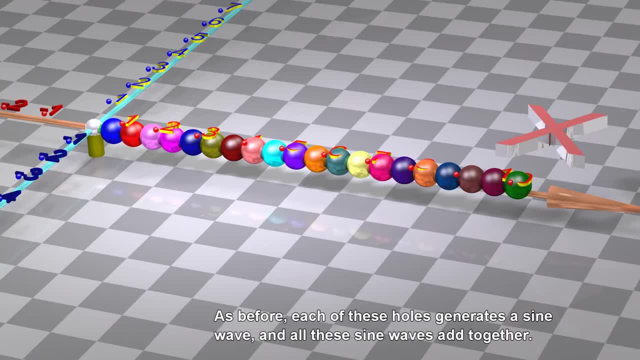 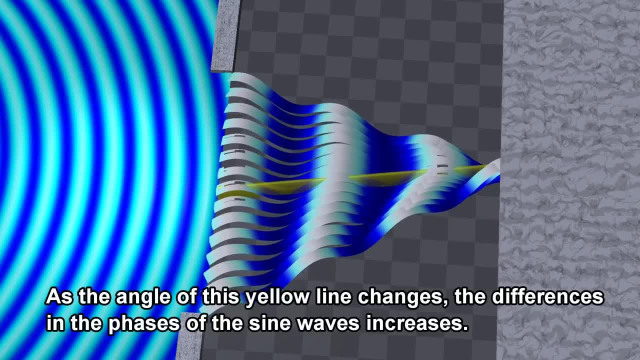 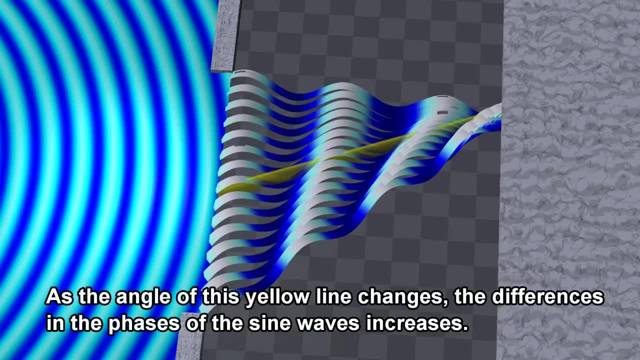